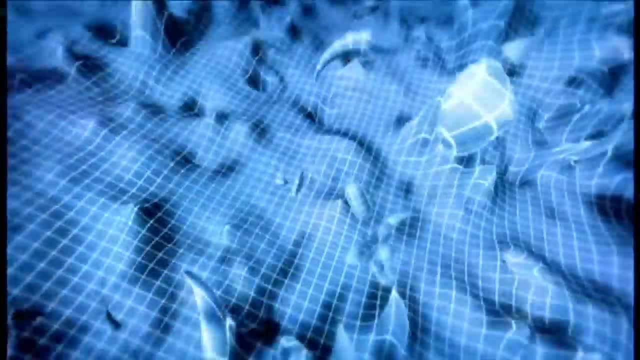 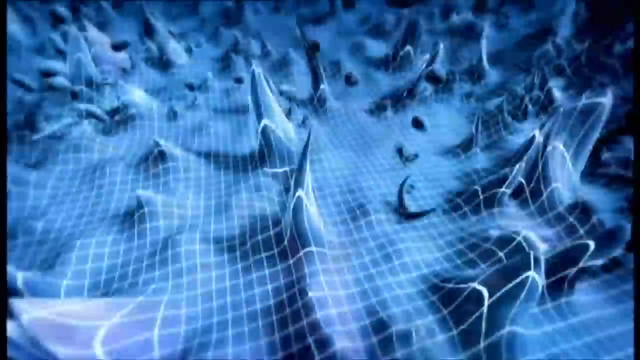 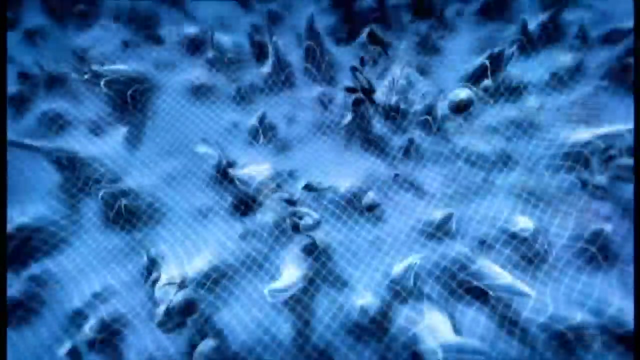 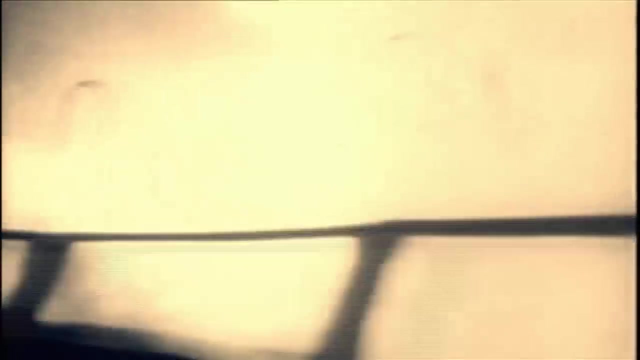 it might be possible to produce a new state of matter that followed quantum rules. It would not be a solid or liquid or gas. It was given a name almost as strange as its properties: A Bose-Einstein condensate For the next 70 years. people could only dream about making such a condensate, which has never been seen in nature. 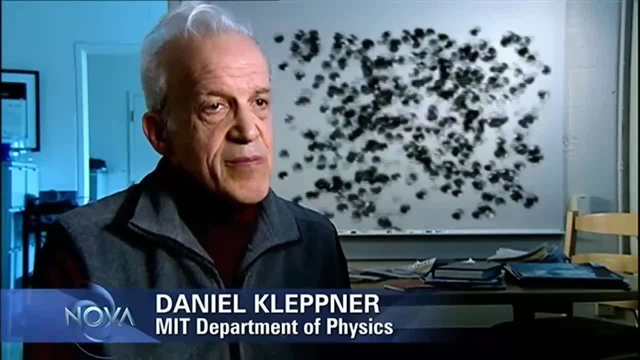 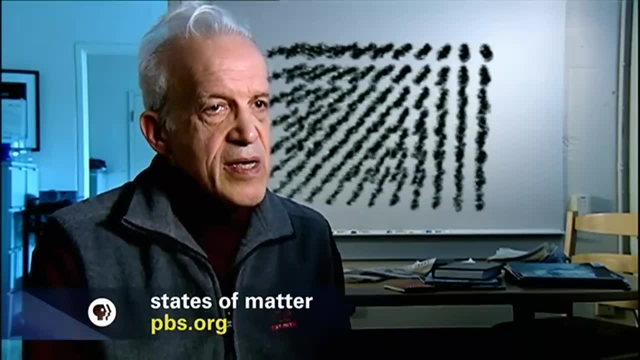 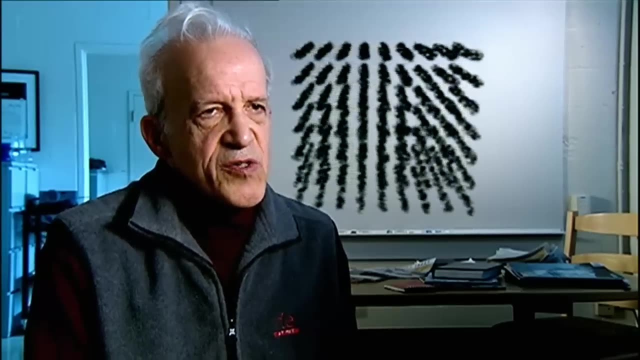 Matter can exist in various states. Atoms at high temperature always form gases. If you cool the gas, it becomes a liquid. If you cool the liquid, it becomes a solid. But under certain circumstances, if you cool atoms far enough to extremely low temperatures, they undergo a very strange transformation. 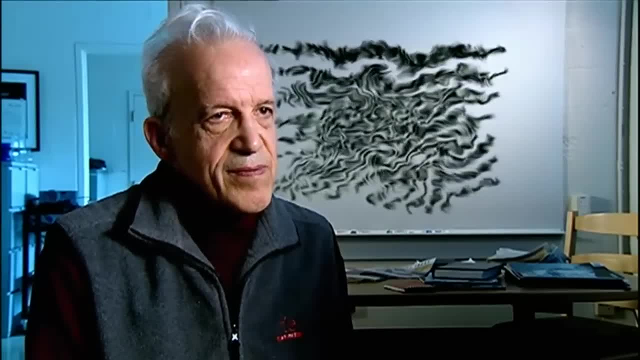 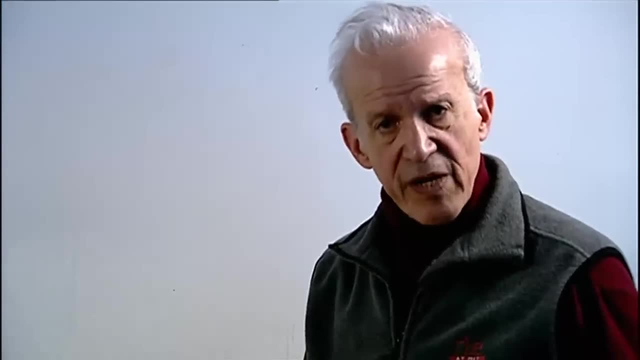 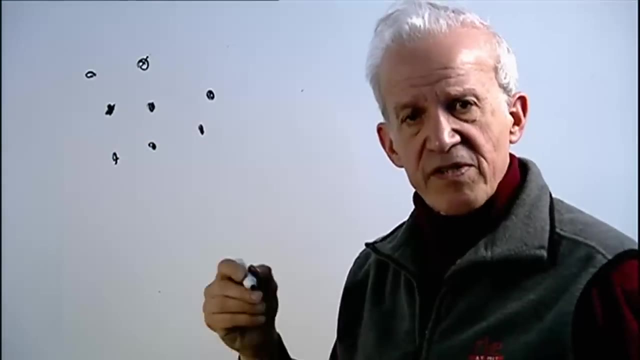 They undergo an identity crisis. So let me show you what I mean by an identity crisis. When you go to low temperatures, the quantum mechanical properties of the atoms become important. These are very strange, very unfamiliar to us, But in fact, each one of these atoms starts to display wave-like properties. 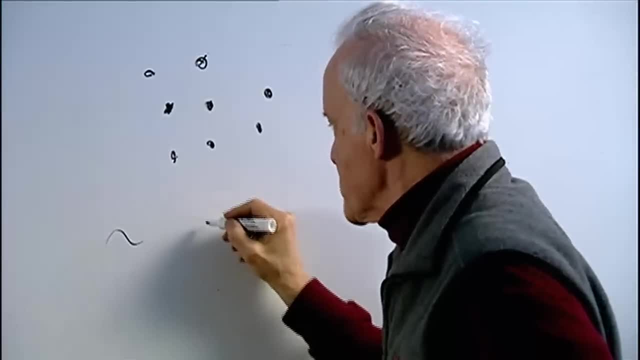 So, instead of points like that, you have little wave packets like that moving around. So, instead of points like that, you have little wave packets like that moving around. So, instead of points like that, you have little wave packets like that moving around. It's really difficult for me to explain why. It's really difficult for me to explain why, But it's the way that it is. Now, as you go to very low temperatures, the size of these packets gets longer and longer, And then suddenly, if you get them cold enough, they start overlapping. 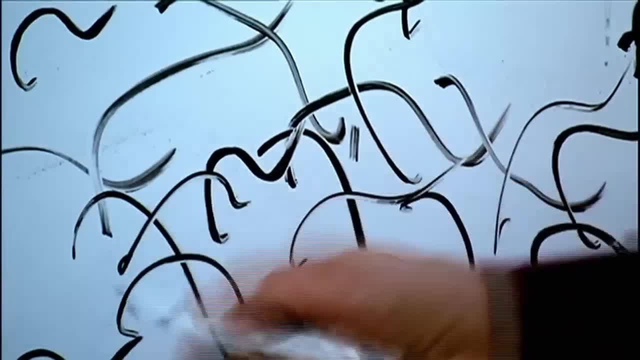 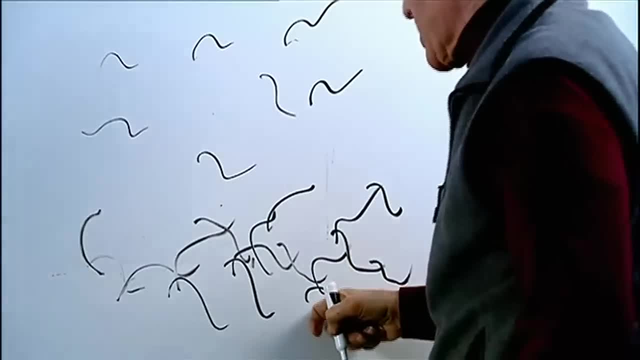 And when they do, the system behaves not like individual particles, but like particles which have left their identity. They all think they're everywhere. This little wave packet over here is known to maintain that shape, This little wave packet over here. 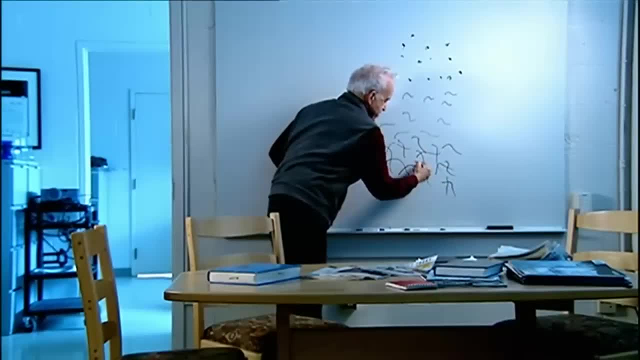 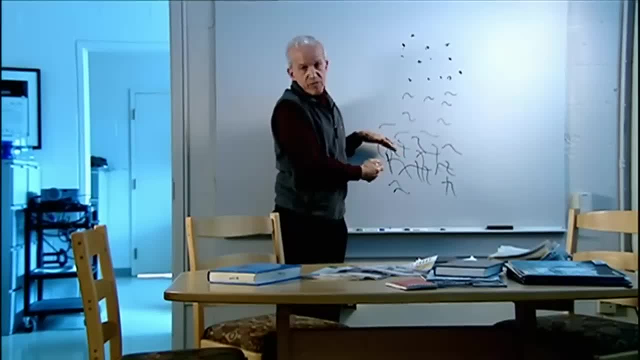 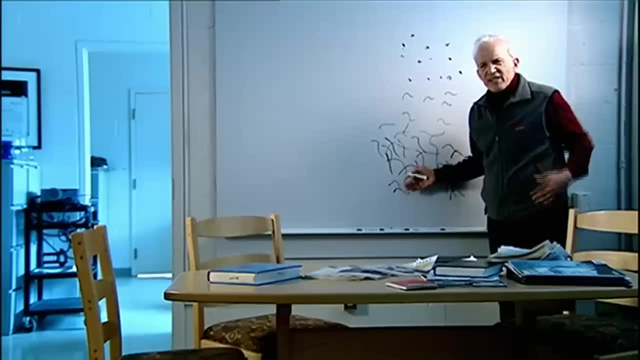 They're all doing the same thing, And what they're doing to a good approximation is they're simply sitting at rest. This Bose-Einstein condensate is very difficult to imagine or to visualize. I can imagine what it's like to be an atom running around gaily freely, bouncing into things. 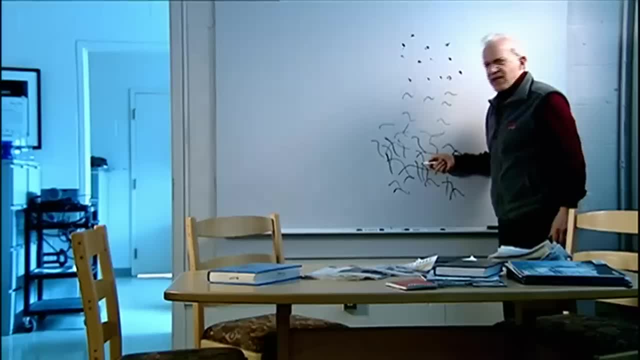 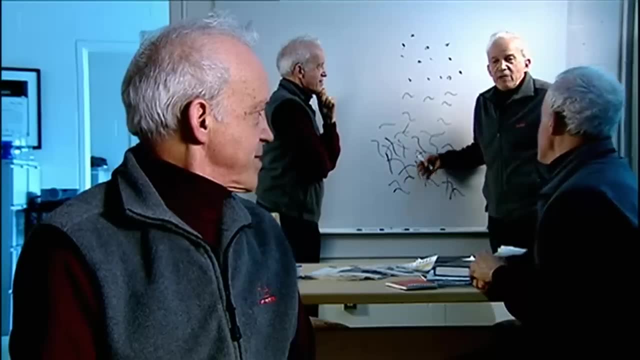 sometimes going fast, sometimes going slow, But on the Bose condensate I'm everywhere at once. I've lost my identity. I don't know who I am anymore. I'm at rest and all the other atoms around at rest.